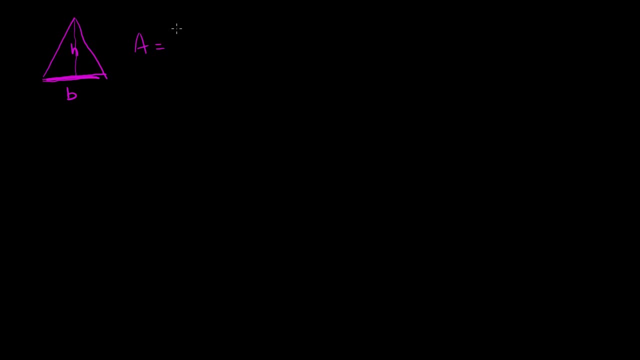 it's pretty common knowledge that the area of this triangle is going to be equal to 1 half times the base times the height. So, for example, if the base was equal to 5, and the height was equal to 6,, then our area would be 1 half times 5 times 6,. 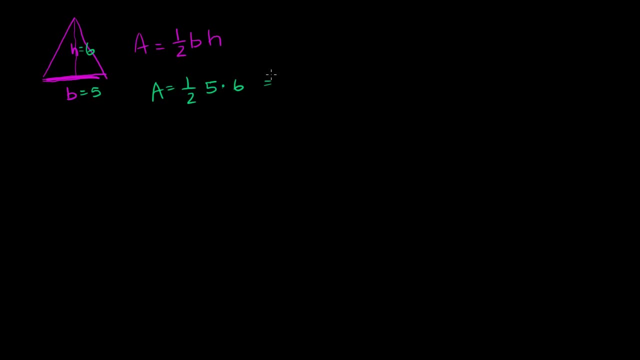 which is 1 half times 30,, which is equal to 15.. Now, what is less well known is how to figure out the area of a triangle when you're only given the sides of the triangle, when you aren't given the height. 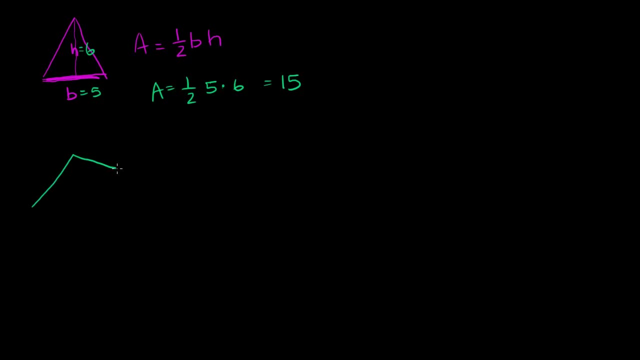 So, for example, how do you figure out a triangle where I just give you you the lengths of the sides? Let's say that side a, side b and side c- a, b and c are the lengths of these sides. How do you figure that out? 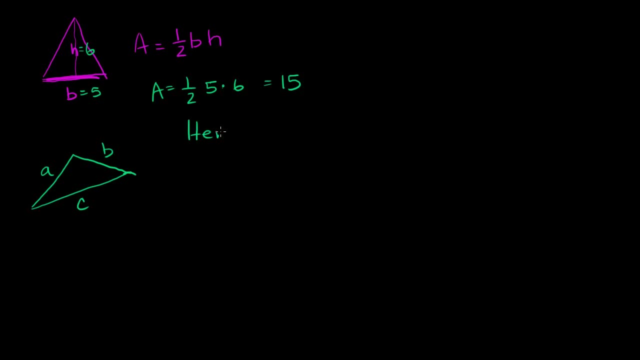 And to do that, we're going to apply something called Heron's formula, And I'm not going to prove it in this video. I'm going to prove it in a future video And really to prove it, you already probably have the tools necessary. 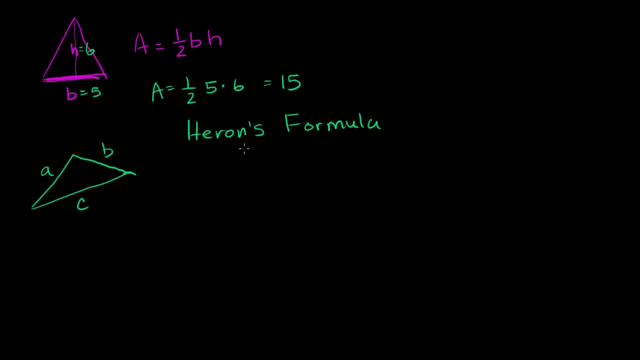 It's really just the Pythagorean theorem and a lot of hairy algebra, But I'm just going to show you the formula now and how to apply it, And then you'll hopefully appreciate that it's pretty simple and pretty easy to remember And it can be a nice trick to impress people with. 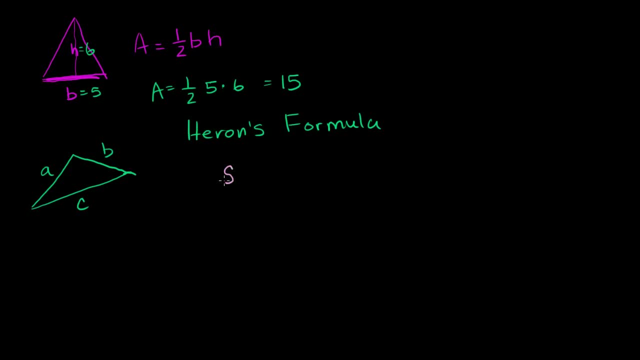 So Heron's formula says: first figure out this third variable, s, which is essentially the perimeter of this triangle divided by 2.. a plus b plus c divided by 2.. Then, once you figure out s, the area of your triangle, of this triangle, right there. 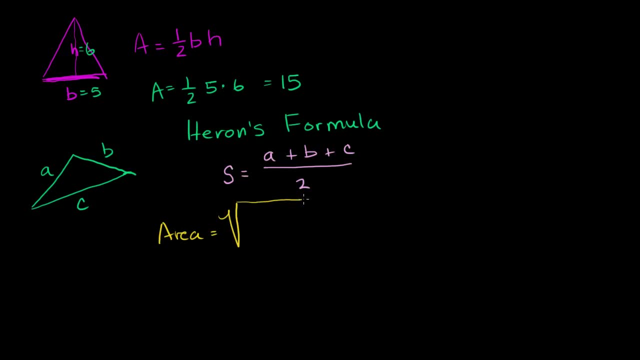 your area is going to be equal to The square root of s. This variable s right here that you just calculated: Times s minus a, times s minus b, times s minus c. That's Heron's formula. right there, this combination. Let me square it off for you. 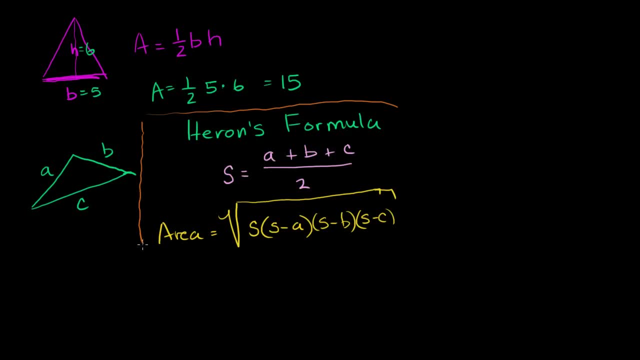 So that, right, there is Heron's formula, And if that looks a little bit daunting, it is a little bit more daunting, clearly, than just 1 half times Base times height. Let's do it with an actual example or two and actually see that it's actually not so bad. 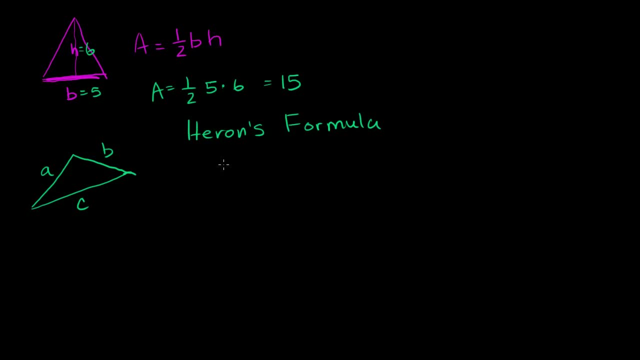 simple and pretty easy to remember And it can be a nice trick to impress people with. So Heron's formula says: first figure out this third variable, S, which is essentially the perimeter of this triangle divided by 2.. A plus B plus C, divided by 2.. 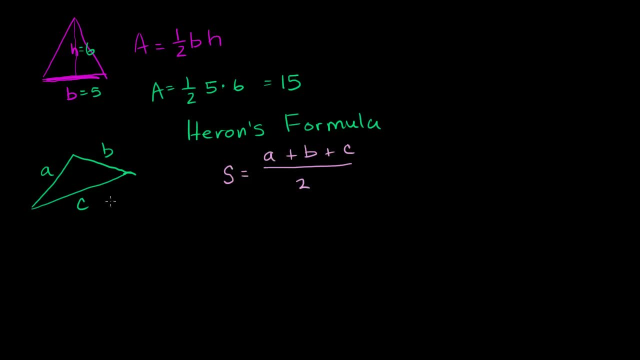 Then, once you figure out S the area of your triangle, of this triangle, right there, your area is going to be equal to this: The square root of S, this variable S, right here, that you just calculated times S minus A, times S minus B, times S. 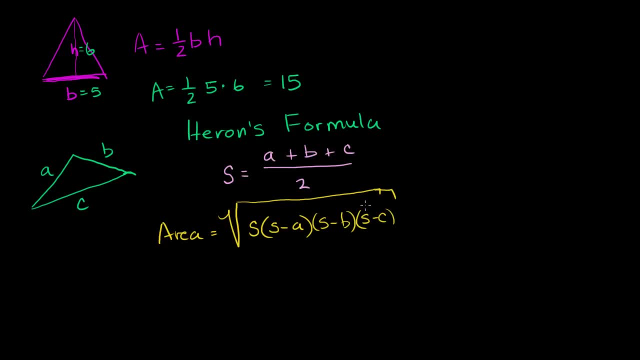 minus C. That's Heron's formula. right there, this combination. Let me square it off for you, So that right there is Heron's formula, And if that looks a little bit daunting, it is a little bit more daunting, clearly, than just 1 half times B squared. 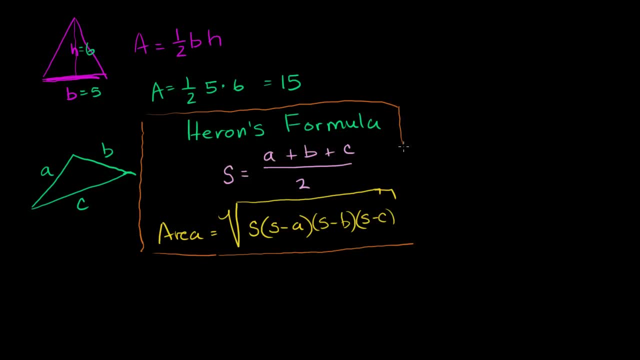 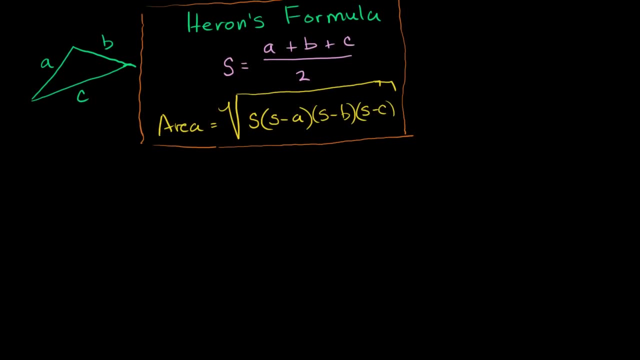 Let's do it with an actual example, or 2, and actually see that it's actually not so bad. So let's say I have a triangle. I'll leave the formula up there. So let's say I have a triangle that has sides of length 9,, 11,. 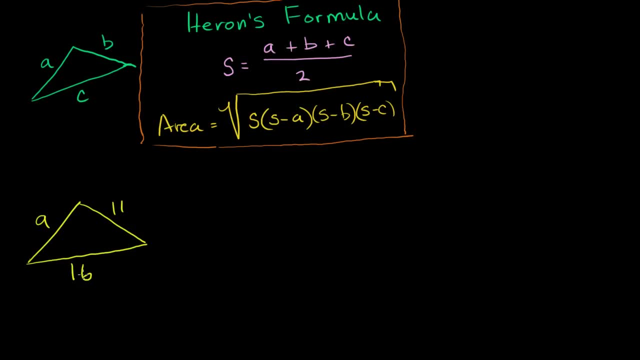 and 16.. So let's apply Heron's formula S in this situation is going to be the perimeter divided by 2.. So 9 plus 11.. Plus 16.. 16 divided by 2, which is equal to 9 plus 11, is 20.. 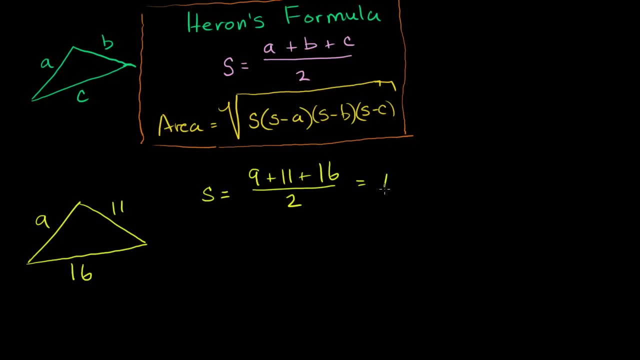 Plus 16 is 36.. Divided by 2 is 18.. And then the area by Heron's formula is going to be equal to the square root of S, 18, times S minus A, S minus 9.. 18 minus 9.. 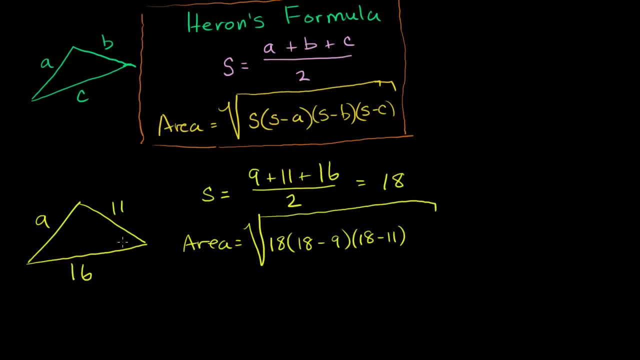 Times 18 minus 9.. S minus 11.. Times 18 minus 16.. 18 minus 16, and then this is equal to the square root of 18 times 9, times 7, times 2.. Which is equal to, let's see, 2 times 18 is 36.. 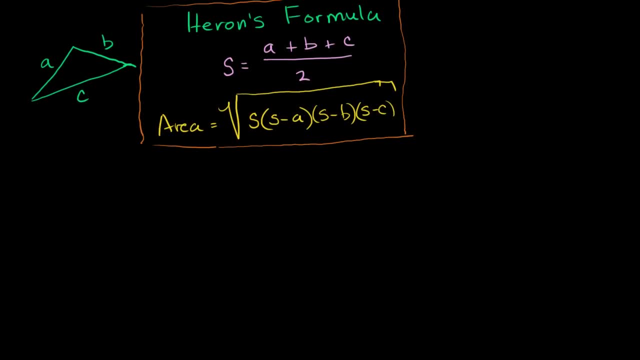 So let's say I have a triangle. I'll leave the formula up there. So let's say I have a triangle that has sides of length 9,, 11, and 16.. So let's apply Heron's formula s in this situation is going to be the perimeter divided by 2.. 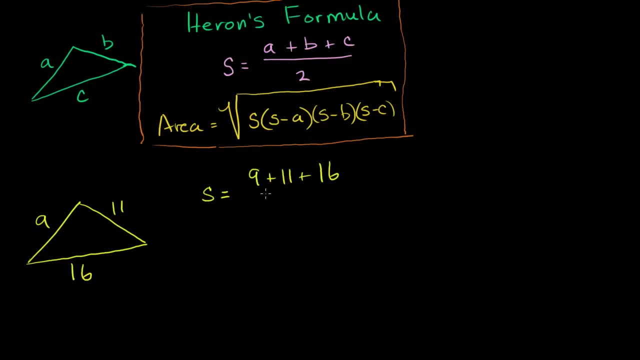 So 9 plus 11 plus s 16, divided by 2. Which is equal to 9 plus 11, is 20.. Plus 16 is 36.. Divided by 2 is 18.. And then the area by Heron's formula. 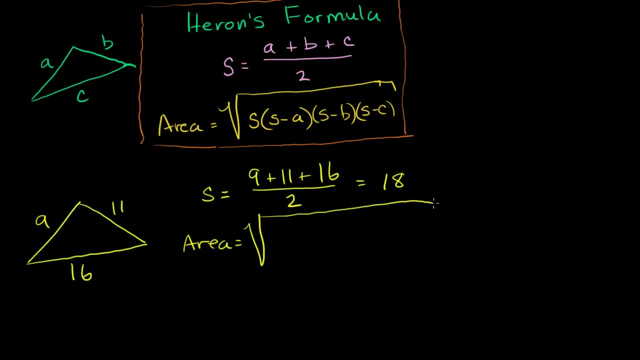 is going to be equal to the square root of s 18. Times s minus a, s minus 9.. 18 minus 9.. Times: 18 minus 9.. Minus 11.. Times: 18 minus 16.. 18 minus 16.. 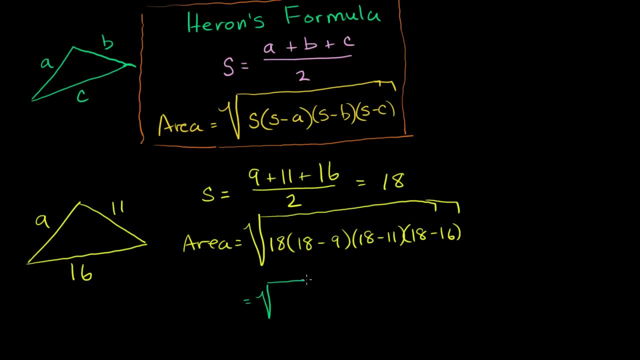 And then this becomes: this is equal to the square root of 18 times 9 times 7 times 2.. Which is equal to, let's see, 2 times 18 is 36.. I'll just rearrange it a bit. 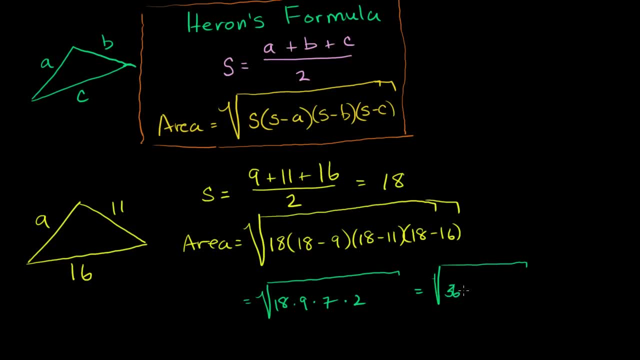 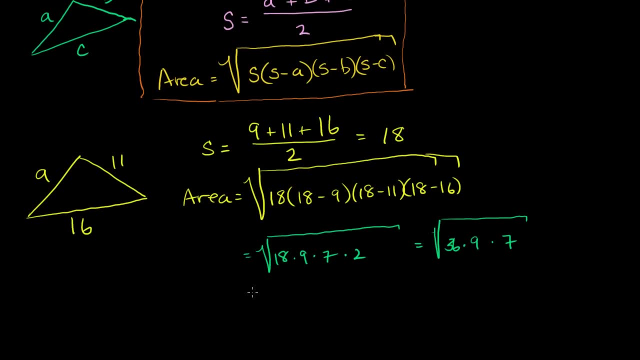 This is equal to the square root of 36 times 9.. Times, 7.. Which is equal to. which is equal to. this is equal to the square root of 36.. Times, the square root of 9.. Times, the square root of 7.. 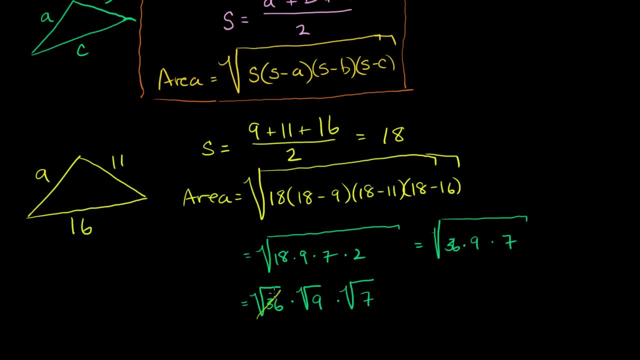 The square root of 36 is just. this is just 6.. This is just 3.. I mean, you don't deal with the negative square roots, because you can't have negative side lengths, And so this is going to be equal to 18.. 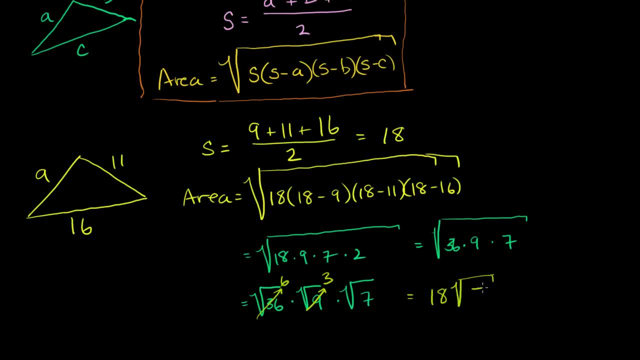 Times the square root of 7.. So, just like that, you saw, it only took a couple of minutes to apply Heron's formula, or even less than that to figure out that the area of this triangle, right here the area, is equal to 18 square roots of 7.. Anyway, hopefully you found that pretty neat. 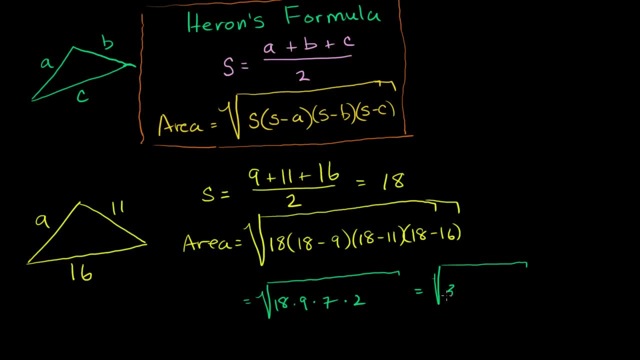 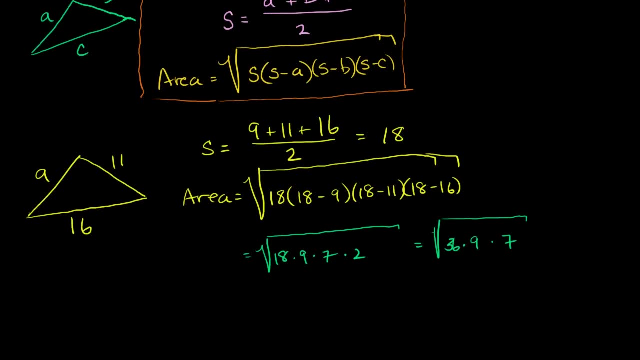 So I'll just rearrange it a bit. This is equal to the square root of 36 times 9.. 9 times 7, which is equal to the square root of 36 times the square root of 9 times the square root of 7.. 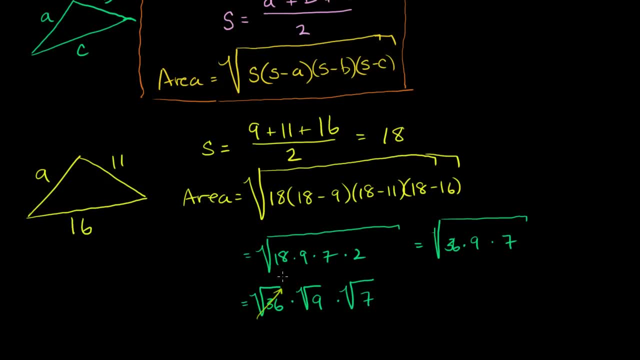 The square root of 36 is just 6.. This is just 3.. I mean, you don't deal with the negative square roots because you can't have negative side lengths, And so this is going to be equal to 18 times the square. 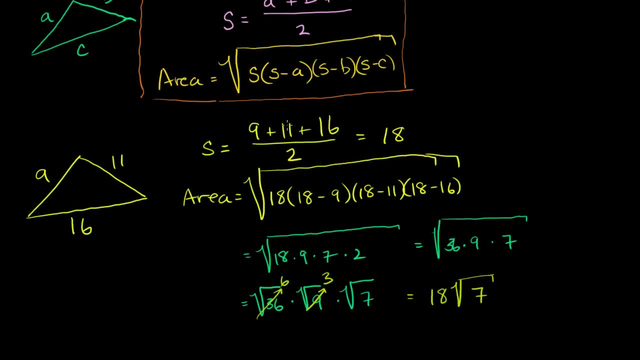 root of 7.. So, just like that, you saw, it only took a couple of minutes to apply Heron's formula, or even less than that to figure out that the area of this triangle right here is equal to 18 square roots of 7.. Anyway, hopefully you found that pretty neat. 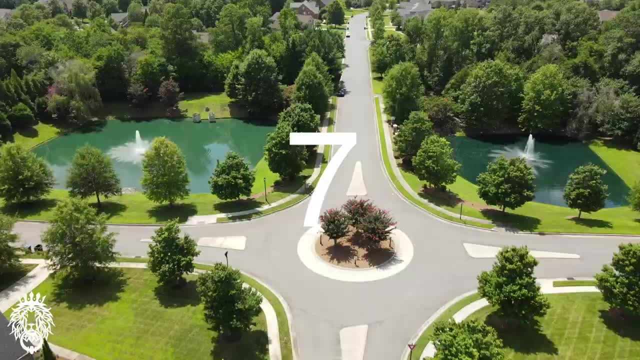 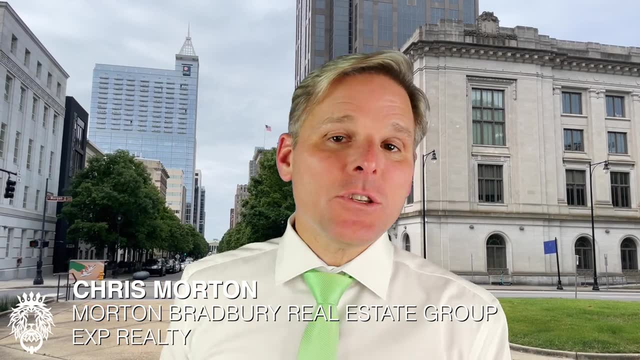 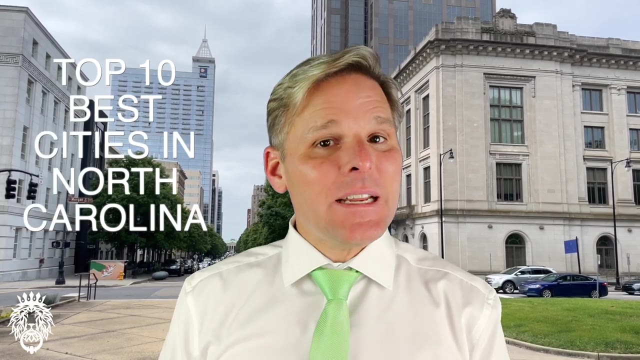 On this video we're going to tell you all about the top 10 highest ranked cities in North Carolina. Hello everyone, This is Chris Morton, real estate broker with EXP Realty in Raleigh, North Carolina, And, as we said, we're going to rank the top 10 best cities in North Carolina. 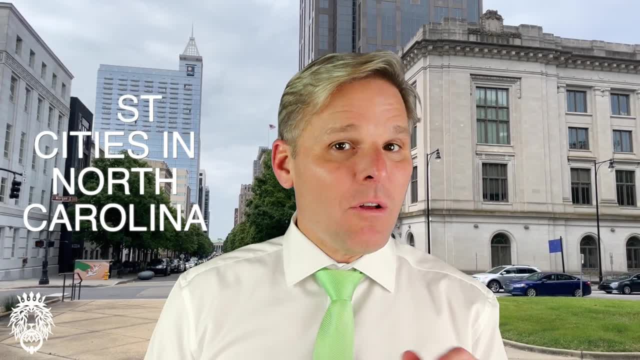 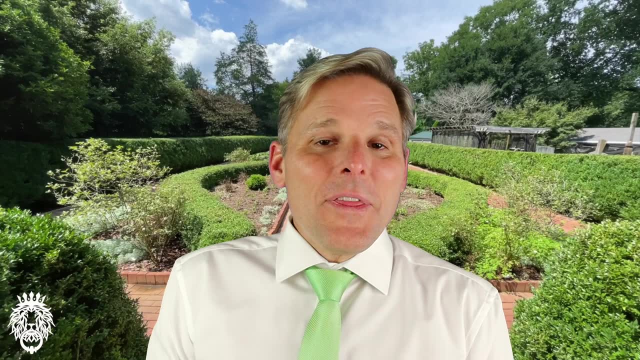 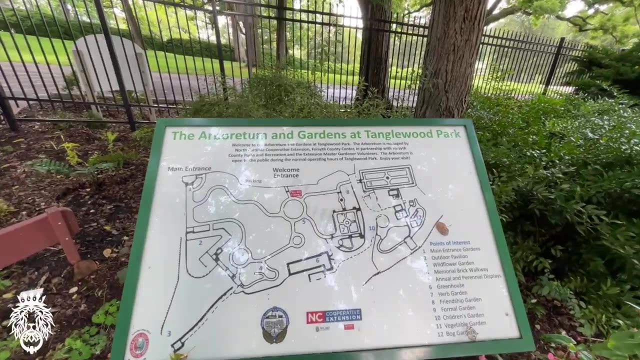 And just a hint, a lot of them are in the Raleigh Triangle area And we should let you know. this list is courtesy of our friends at Nichecom. Let's start with the number 10 city, which is Clemens, North Carolina. Clemens is a suburb of Winston-Salem, North Carolina. It has a population. 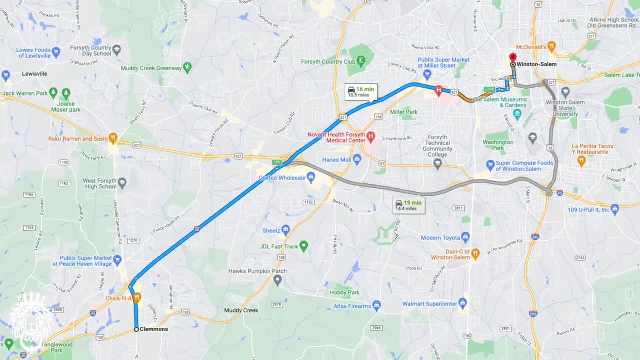 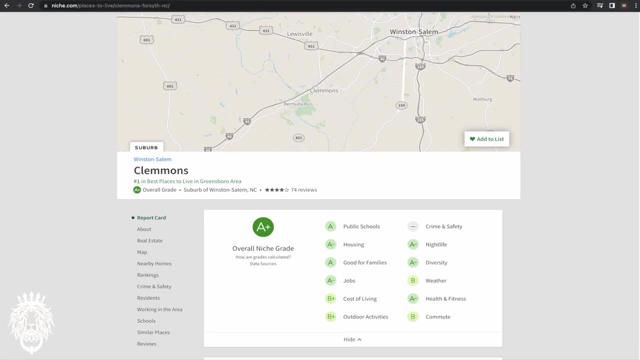 of about 22,000 people. It's about 15 minutes from Winston-Salem And Nichecom gives Clemens an overall rating for the city of an A+. Public schools in Clemens get an A, Housing in Clemens gets an A-. 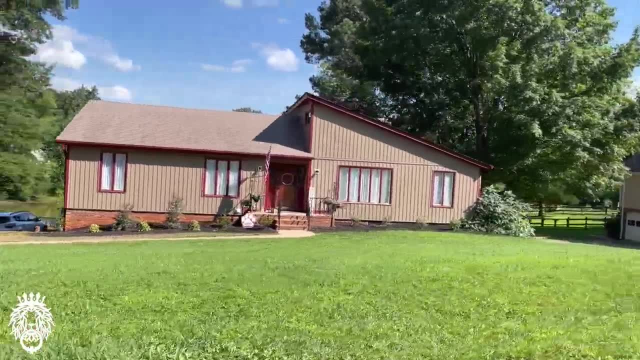 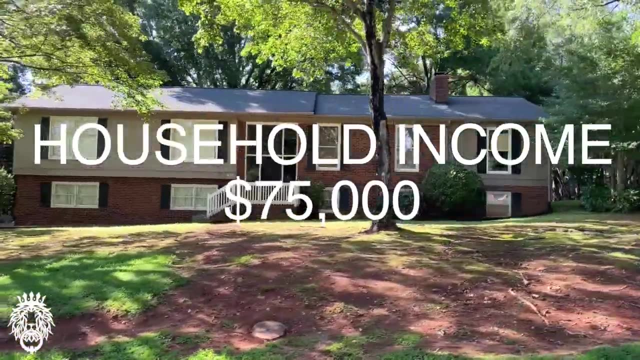 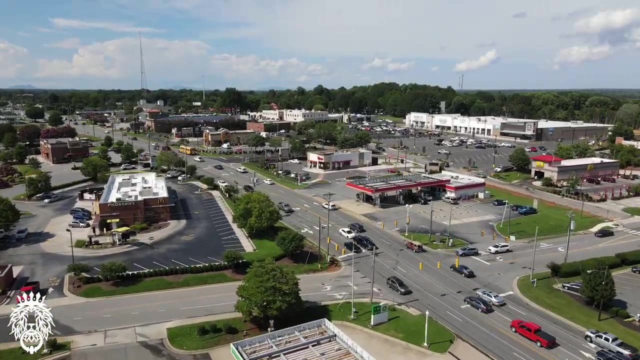 And the median home price for a home in Clemens is $345,000.. Median household income in Clemens comes in at $75,000.. So Clemens doesn't have a whole lot going on in the city proper, but what it does have going for it is that it is really really close to Winston-Salem.